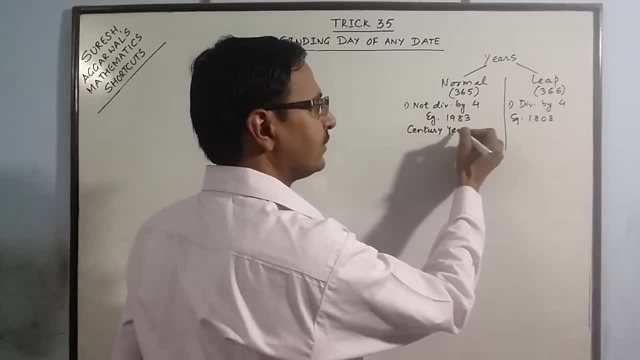 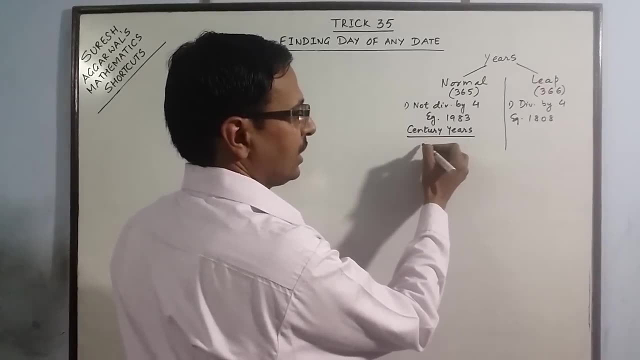 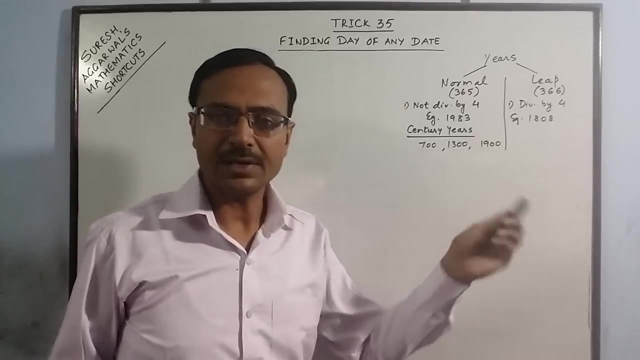 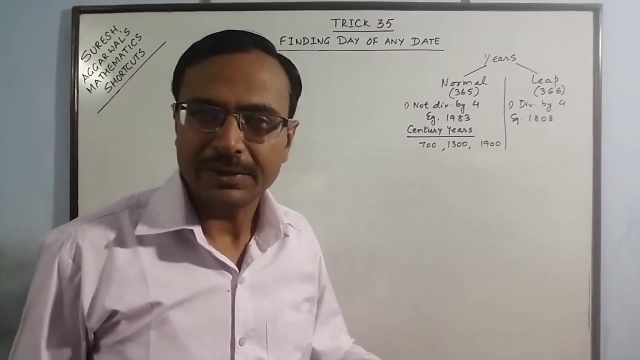 Now, century years are all those years which have two zeros at the end. Say we have 700, 1300, 1900.. All these years are century years And for checking whether a century year is a normal year or a leap year, 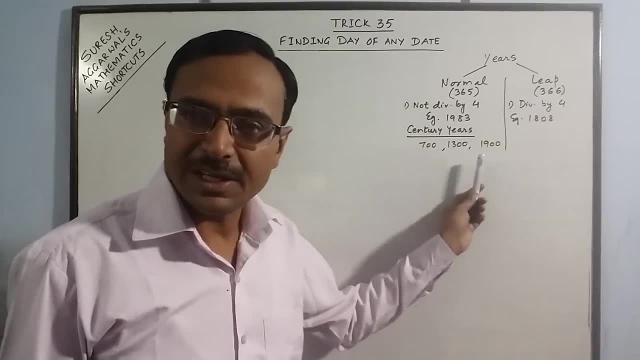 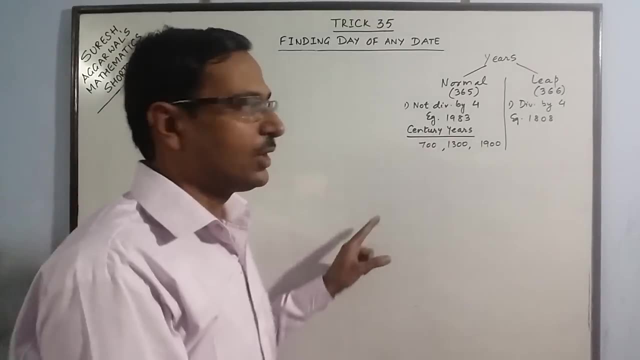 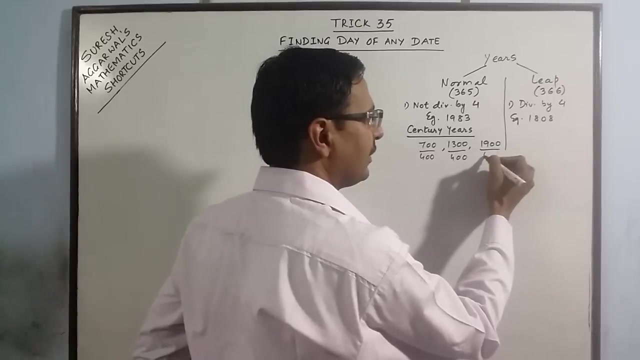 you have to check the divisibility of this year by 400 and not by 4.. Since 700 is not divisible by 400, divisible by 400,. when you divide this by 400, you will get a remainder. So these years, 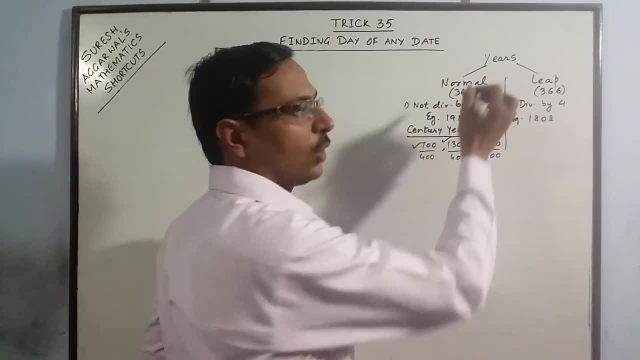 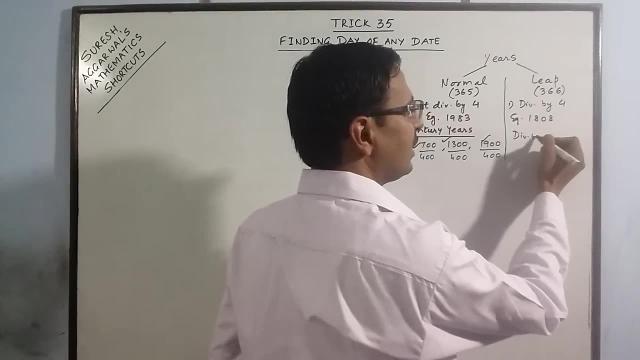 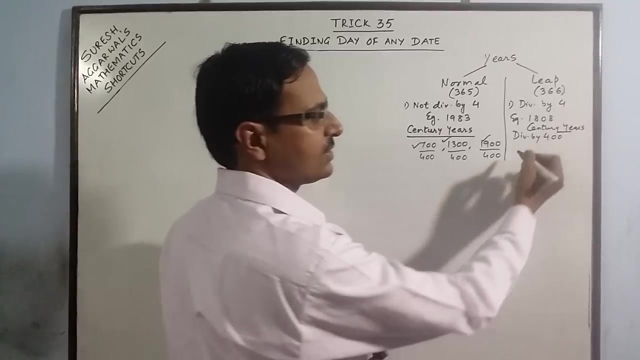 All these years are normal years, Whereas all the century years which are divisible by 400,, in case of century years, years which are divisible by 400,, just like we have 1200, 1600, 2000 and so on. 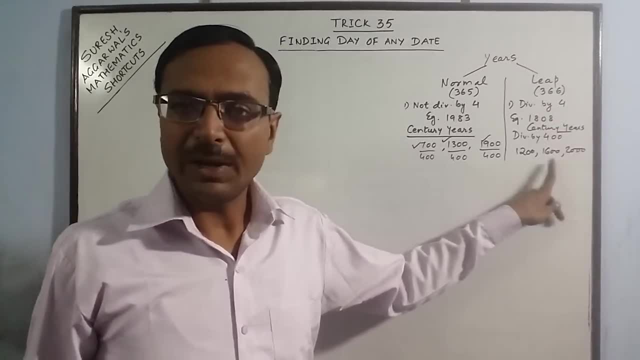 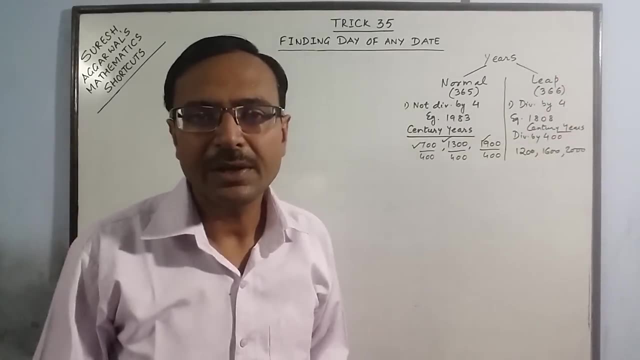 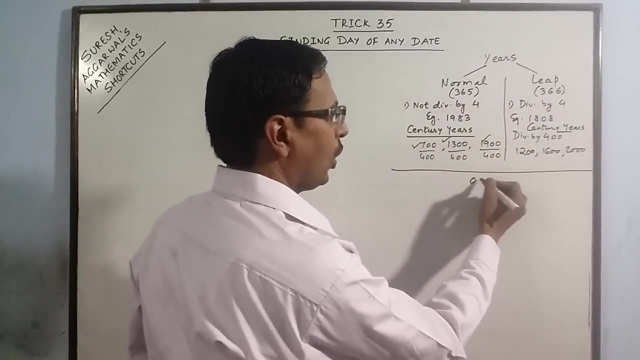 These years are all divisible by 400. So they are also leap years. So now you know which year is a leap year and which year is a normal year. Now coming to the concept of odd days. Now, what are odd days? 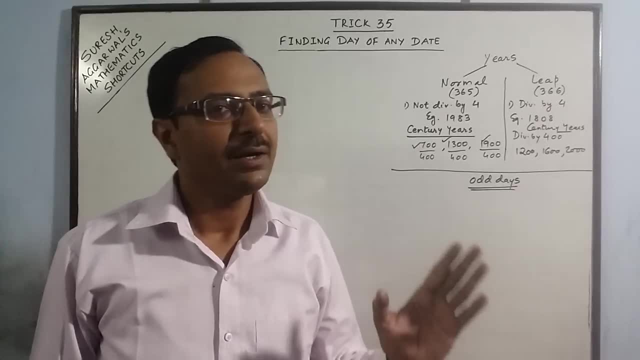 If you understand what are odd days, then half the problem of finding a day of a given day is solved. Odd days Say: we have 365 odd days. We have 325 odd days in the calendar year. For the other days, we have 325 odd days. 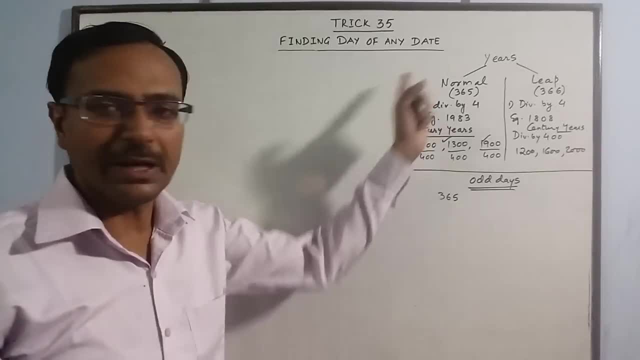 For the other days, we haveépіль of odd days, And then we have a day in the calendar year, days in a year, in a normal year. if you divide this by 7, obviously 7 days in a week. so you get 1 as the remainder. So in a normal year we have 1 odd day, which is excessive means when you divide 365 days into weeks, we will have 1 day left. that is called odd day. In case of a leap year, you have 366 days, and when you divide 366 by 7, you get. 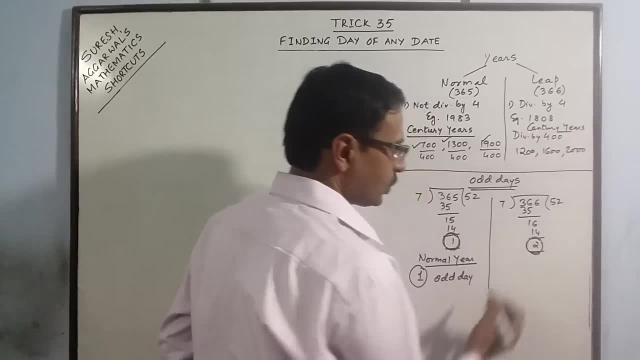 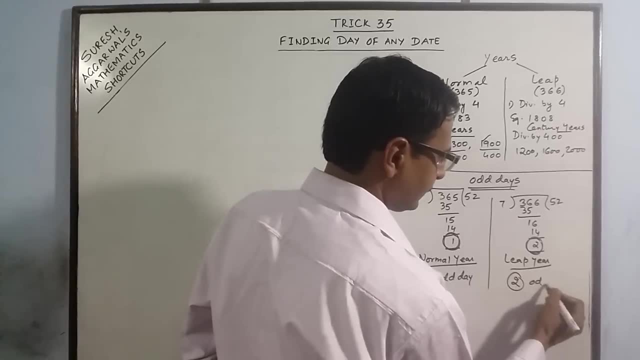 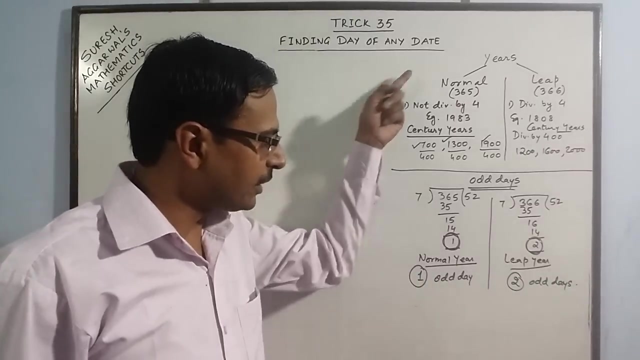 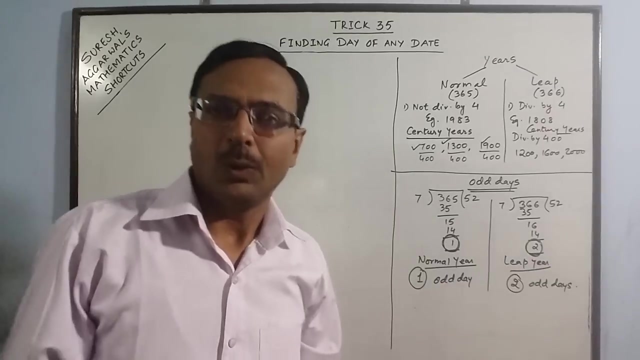 2 as the remainder. So in case of a leap year, you have 2 odd days. So this is very important part of this trick: In a normal year there are 1, there is only 1 odd day, and in a leap year there are 2 odd days. Now coming to the second important 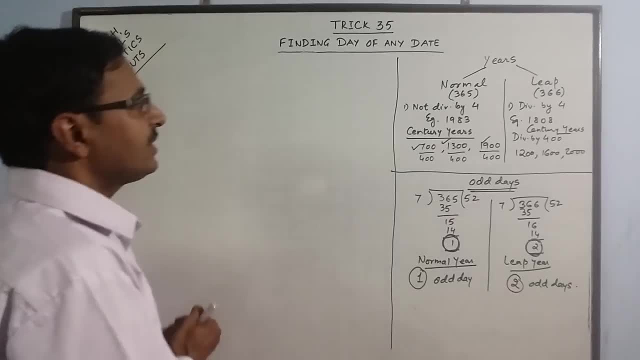 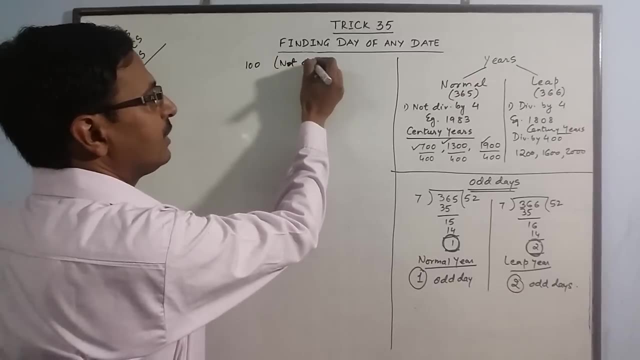 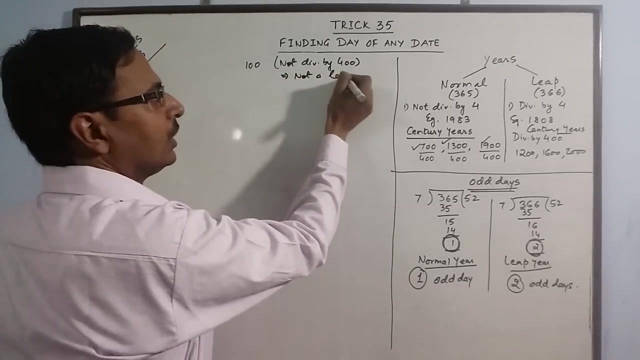 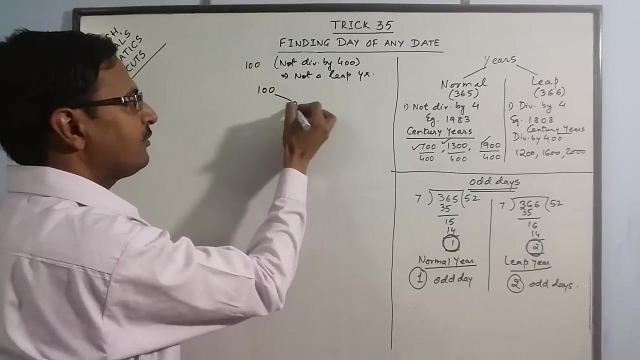 concept concerning this trick 35,, we have the first century year, 100. Now, 100 is not divisible by 400. So it is not a leap year. Now, if it is not a leap year, then in 100 years we have 24 leap. years. When we divide this by 4, we get 25, but that includes 100 also, which is not a leap year. So we get 24 leap years and the remaining 76 normal years. 76 normal years have 1 odd day each, So number of odd days are 2 odd days. So we have 26 normal years. 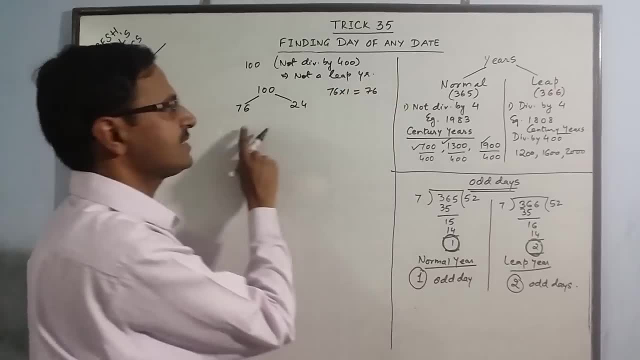 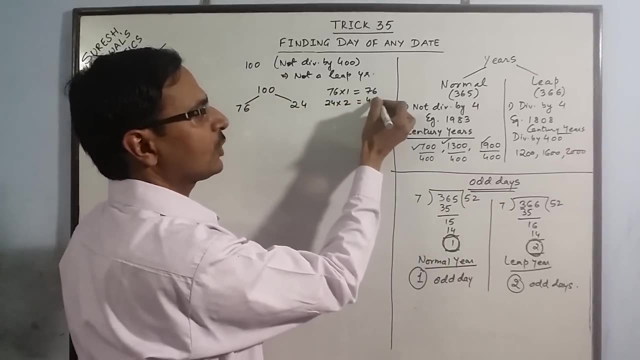 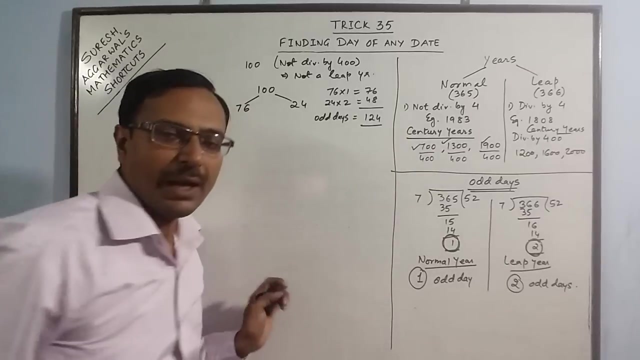 It means that in a normal year we have 36 odd days. days is 76 in these 76 years and leap years have two odd days. So 24 multiplied by 2 that is 48. So total number of odd days in 100 years is 124, and odd days cannot be greater. 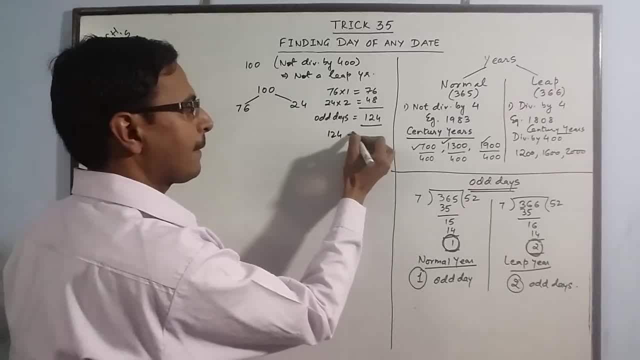 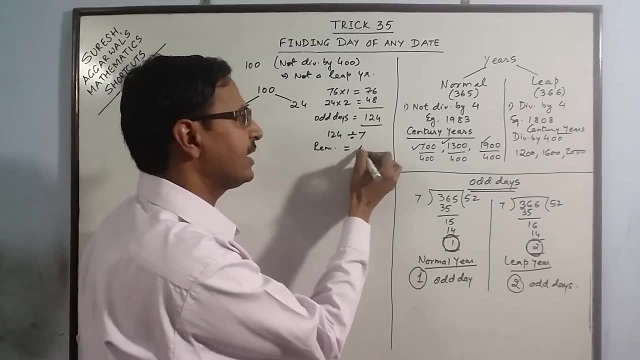 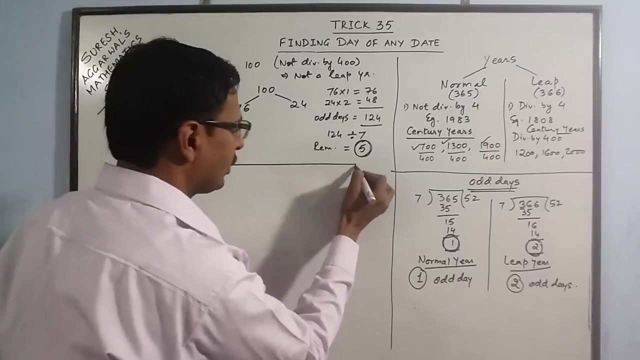 than 7.. So divide 124 by 7 and you get the remainder. as say, 7 x 1 is 7,, 54,, 7 x 7 is 49,, your remainder is 5.. So these are the 5 odd days in 100 years. So we have to remember. 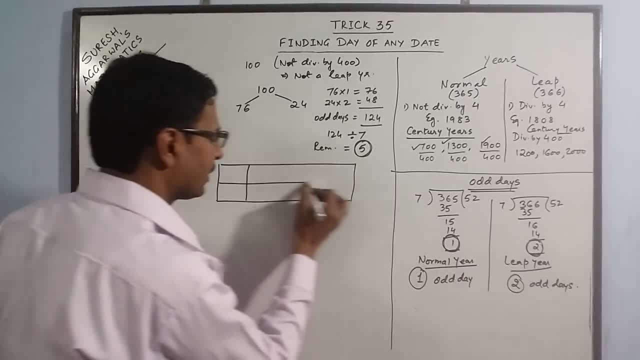 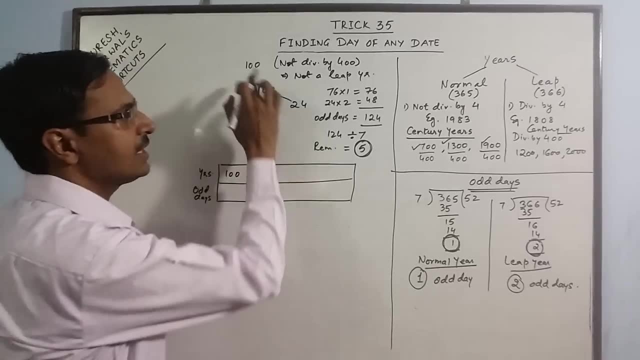 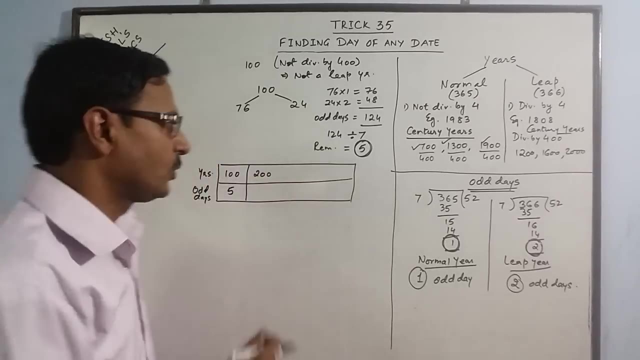 one table here. These are 100 years and these are the odd days. In 100 days, 100 years, you have 5 odd days. Now you can double the number of odd days because 200 is also not a leap year. So 100 have 5 odd days. So you can double the number of odd days because 200. 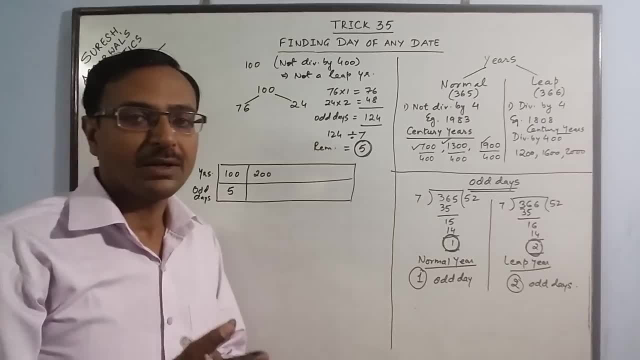 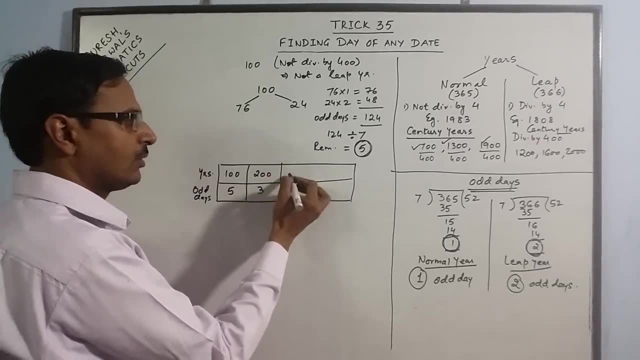 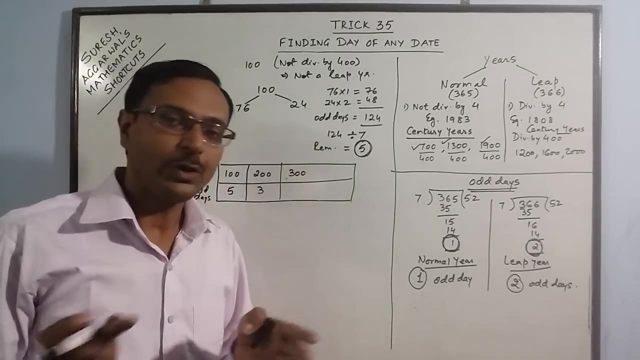 have 5 odd days, So 10, but it cannot be greater than 7.. So 10 can be divided into 7 plus 3.. So 3.. Now coming to the next century: 300, 5 into 3, 15.. So when you divide 15, 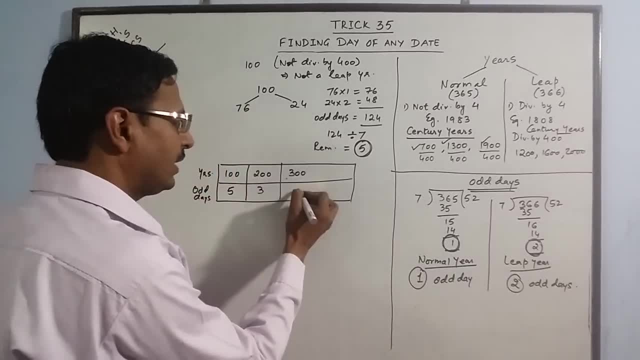 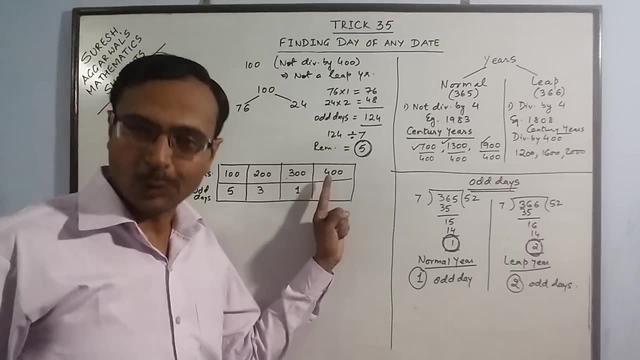 into weeks 7,, 7 and 1. So you get 1.. But when you arrive at 400 years, 400 is divisible by 400.. So this is not a leap year. So this is not a leap year. So this is not a leap. 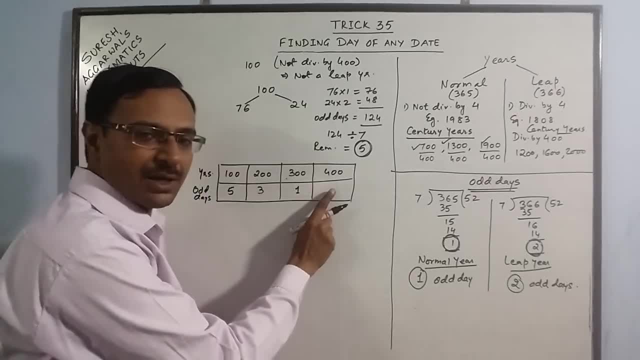 So this is not a leap year. So this is not a leap year. So this is not a leap year. This is a leap year. So 5, fourths are 20 and 400 also is a leap year, So 21.. And when? 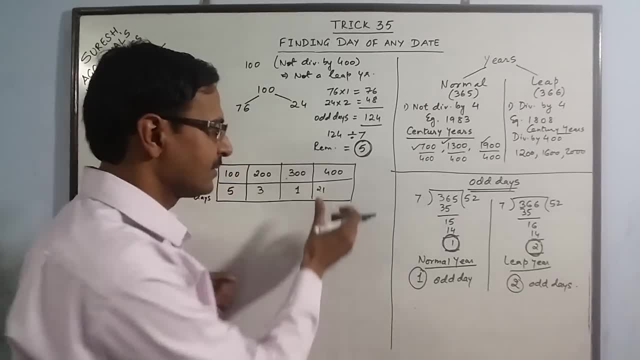 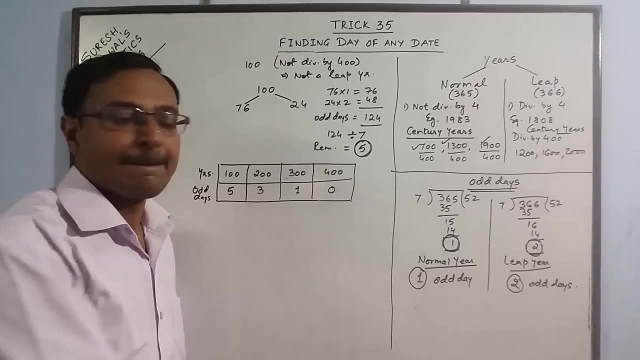 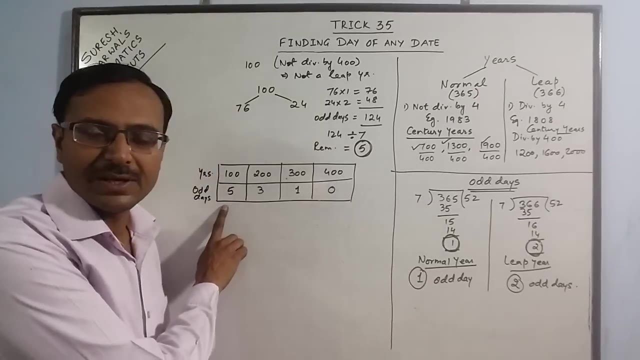 you divide 21 by 7, it is exactly divisible. So there are no odd days. So for 400, there are 0 odd days. So this is another important concept which we have to remember: For every 400 years there are 0 odd days, And then for 100 years we have 5 odd days, 200 years. 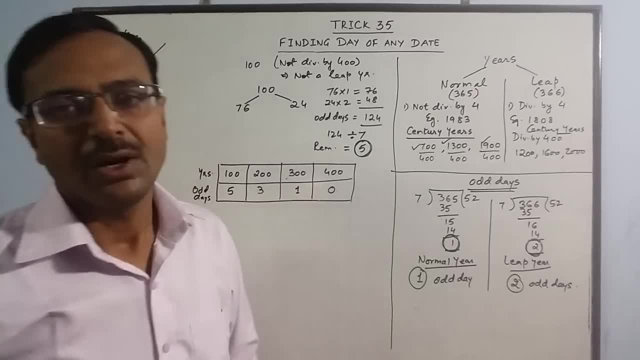 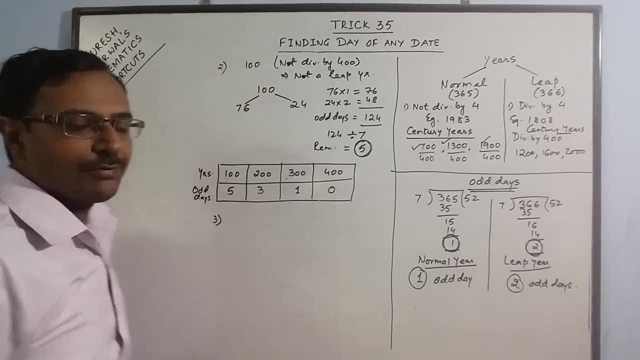 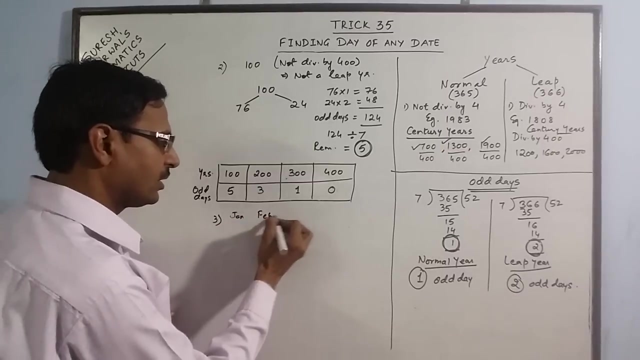 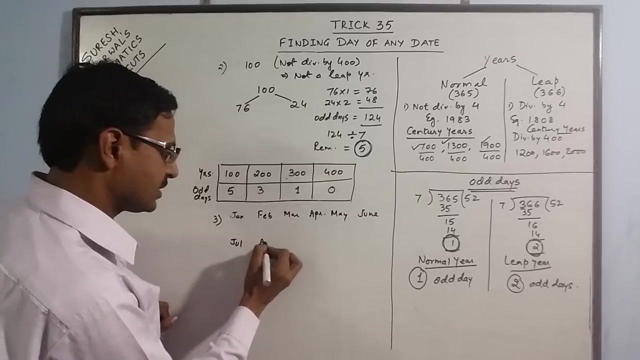 we have 3 odd days For 300 years. we have 1 odd day Now coming to the 3rd important concept of months, As you all know that, starting from January, February, March, April, May, June, July, August, September, October, November and December. You already know the number of months, So you can see 30 rounds of days of these month 31.. Now February. it has either 28 or 29 days, depending on whether it is normal year or a leap year. Then 31,, 30,, 31,, 30, ,31,, 31,, 30,, 31,, 30,31,. 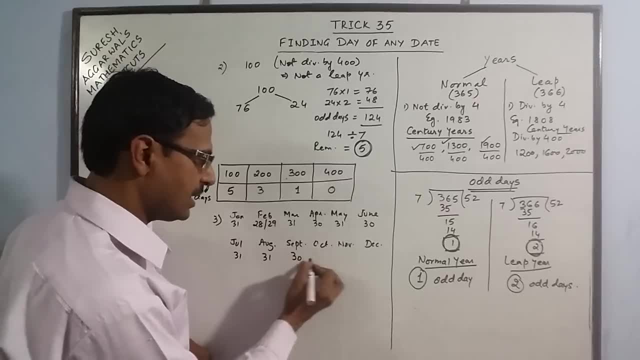 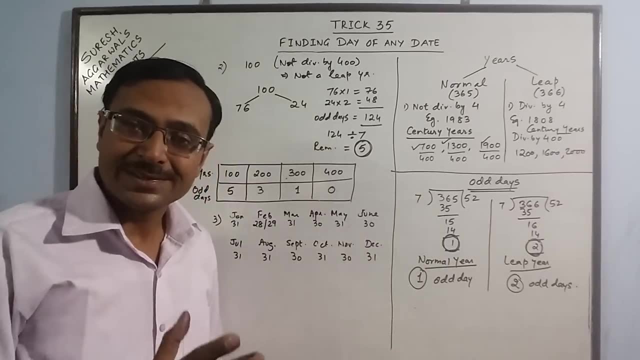 30, 31.. Now, when you divide it into weeks, you will get the number of odd days of every month. So 31 weeks, So 31 checking. Okay, Now, I am not going to spend much time. I am going to discuss it later, Now that we have. 7 x 28,. so you get for 31 days of any month, you get 3 odd days. Why? Because 31 divided by 7 is 28,. 7 x 28 and remaining 3 days are the odd days. Similarly, for 30, 7 x 28 days. 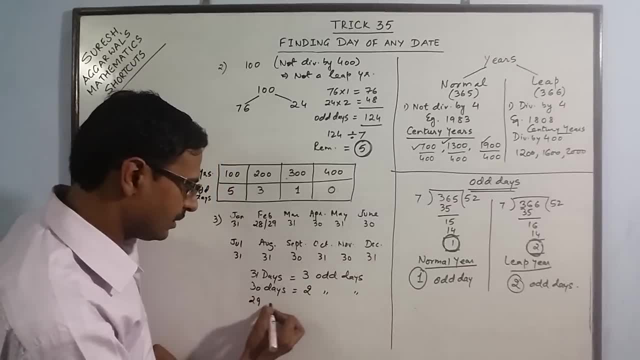 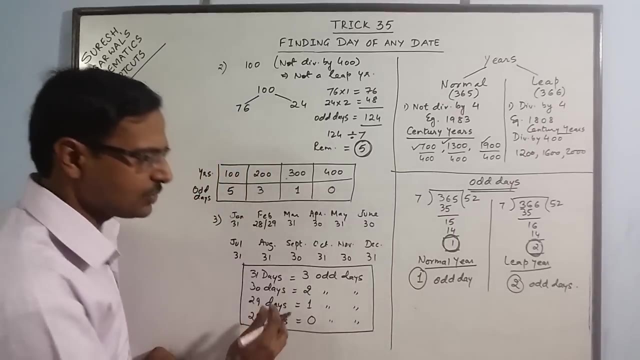 and 2 odd days, For 29, 7 x 28, 1 odd day and for 28,, obviously, 7 x 28, 0 odd days. So this is another important concept which you have to remember. Now we have 3 important 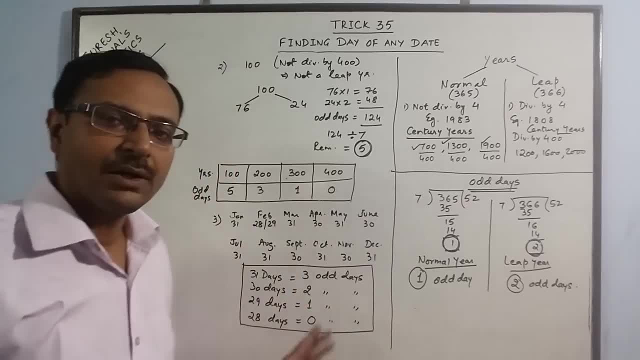 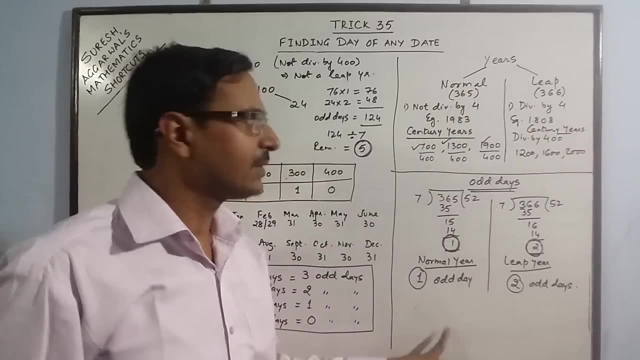 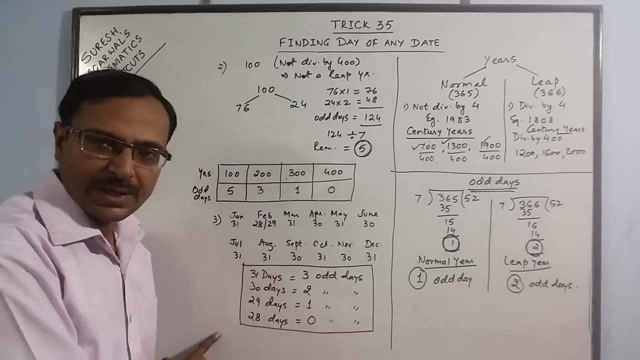 concepts which are to be taken into consideration for finding the day of any date. First is the number of odd days in a normal year and in a lead year. This is the first concept. Second is the century years up to 400, number of odd days in each and then month wise number. 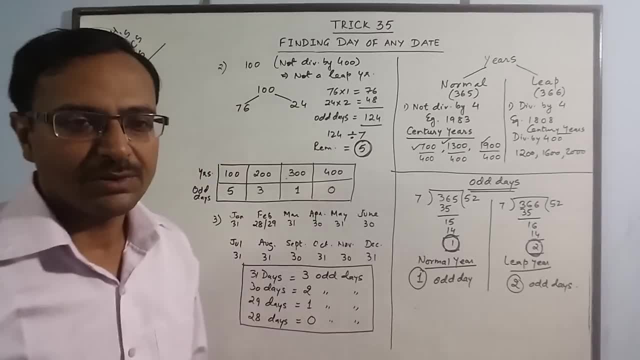 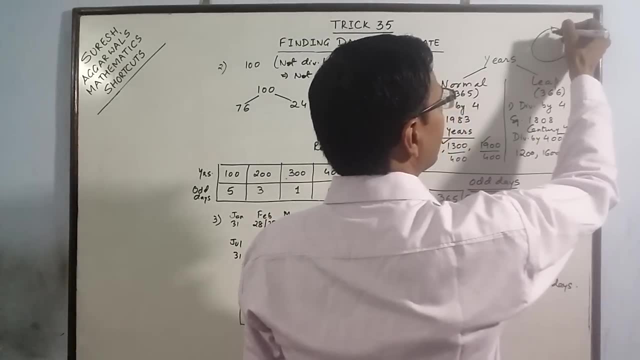 of odd days. Now, the final concept which you have to remember is you have this circle: here We have 0 odd days, 1 odd day, 2 odd day, 3 odd days, 4 odd days, 5 odd days, and. 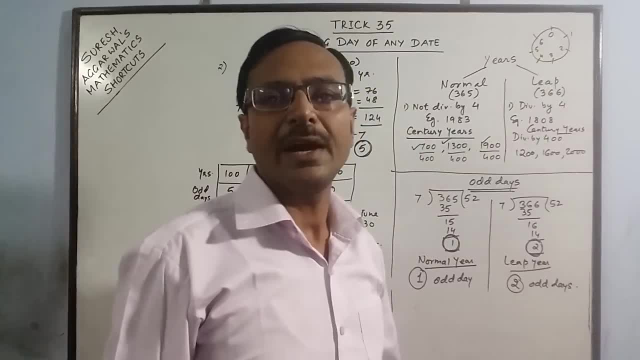 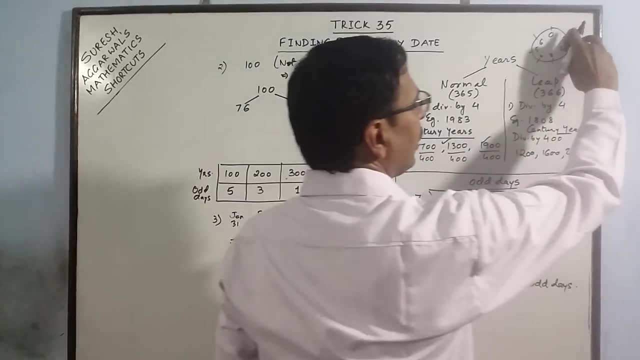 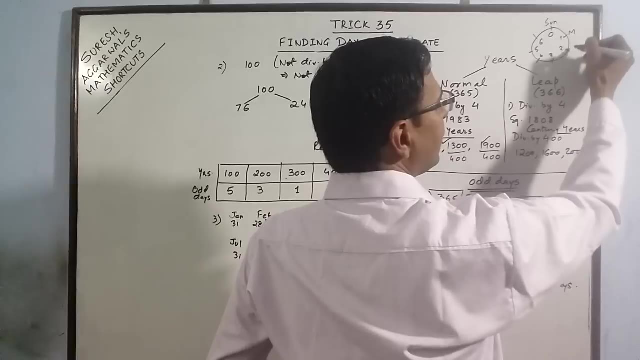 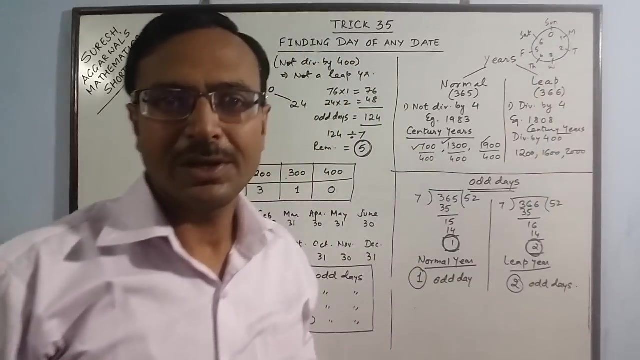 6 odd days: 0 to 6, now we have the days. Now, if there are finally 0 odd days, then the day is Sunday. 1 odd day: Monday, Tuesday, Wednesday, Thursday, Friday and Saturday. So this is the final concept which we have. 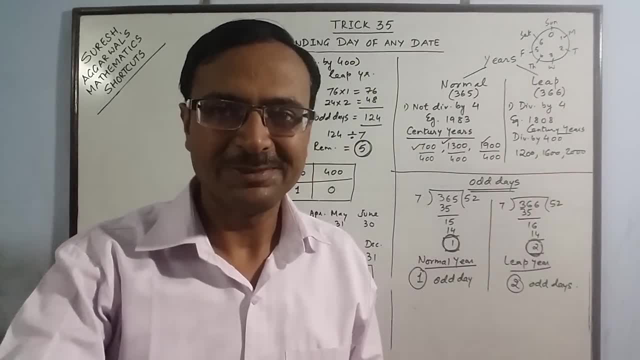 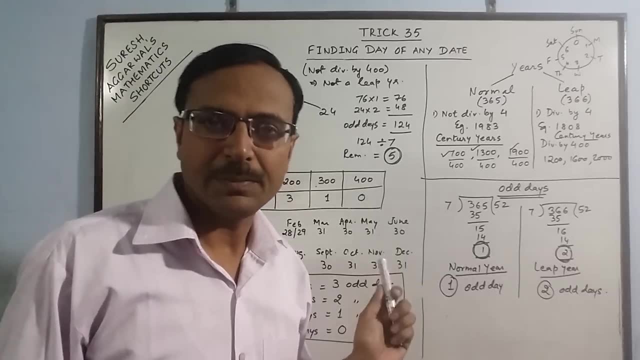 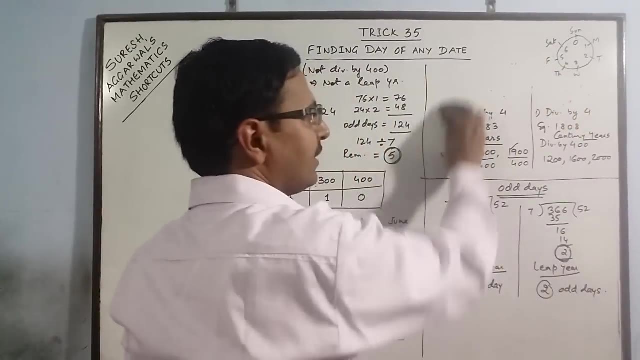 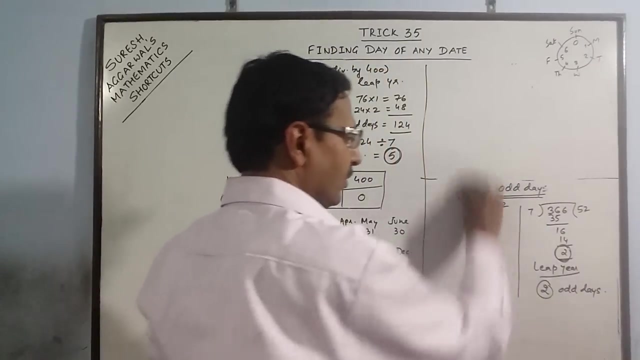 to remember, to find the day of any date. Now let us use these concepts to illustrate the concept by using one or two examples. I will run this off. Let us take one date in which we have a normal year and in the second example we will be taking one date in which it is. 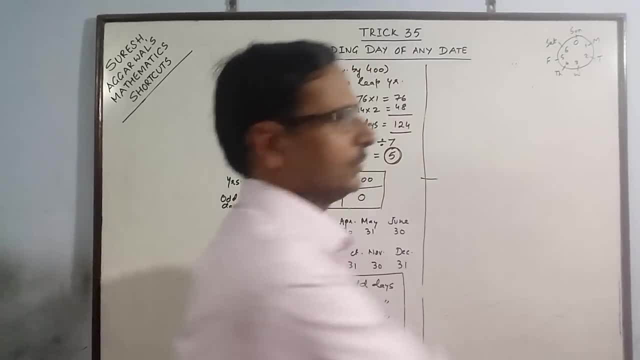 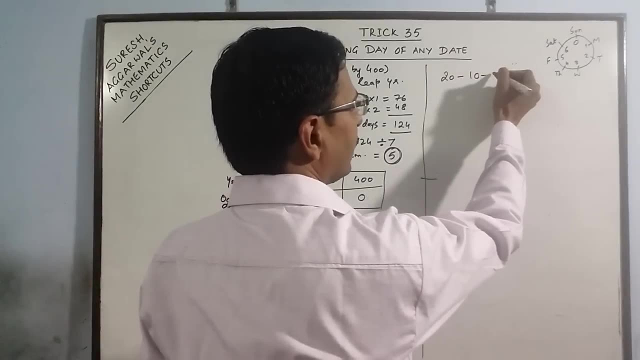 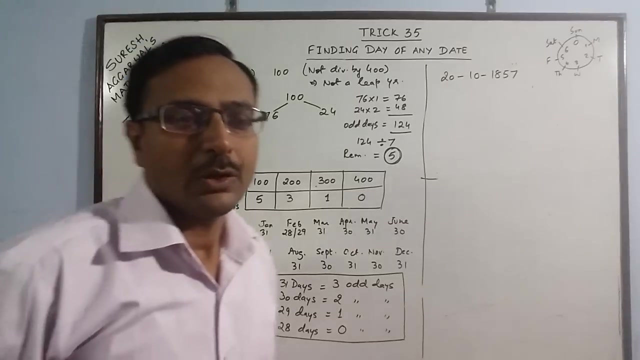 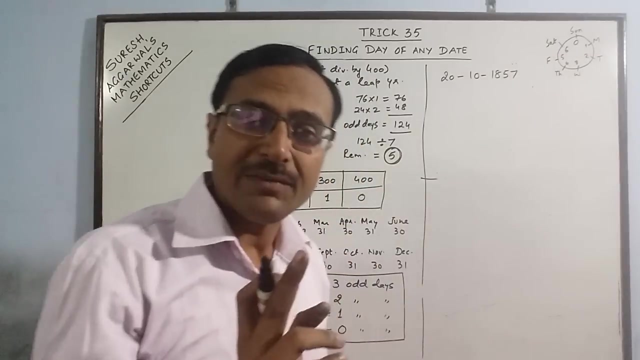 a lead year. Now the first example which I am taking is: say we have 20th October, say we have 1857. Take a different century, 1857. Now the first step is to, because 1857, the year 1857 is. 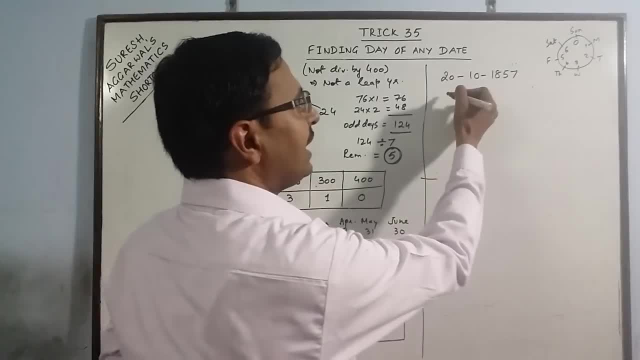 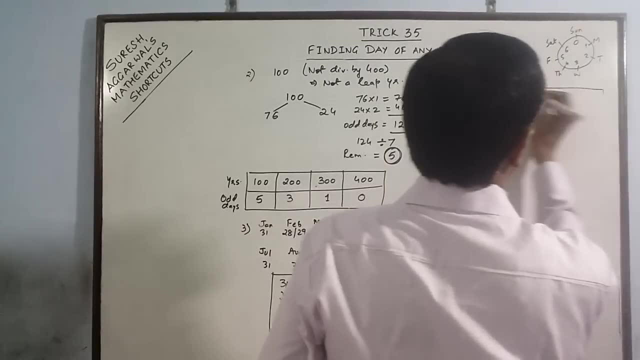 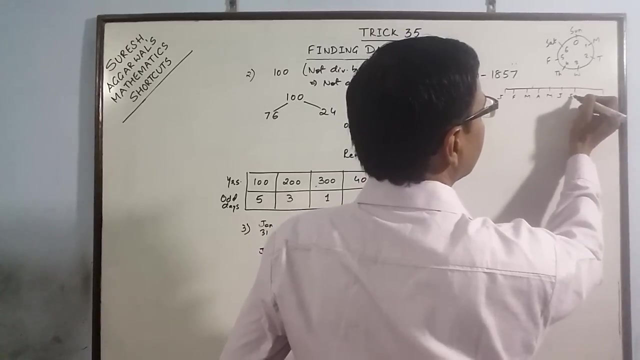 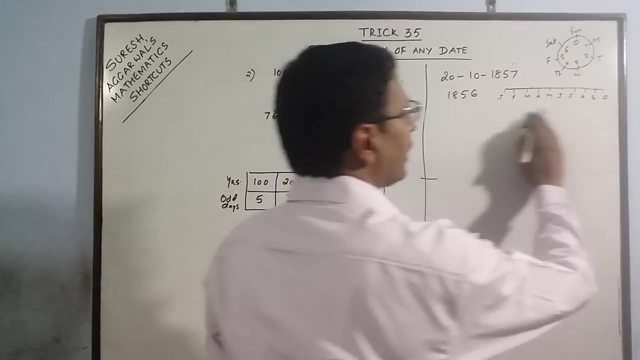 not complete. We have reached up to October only. So we have 1856 complete years and one incomplete year. that is from January, February, March, April, May, June, July, August, September and October. We have up to October, So we have this complete year. 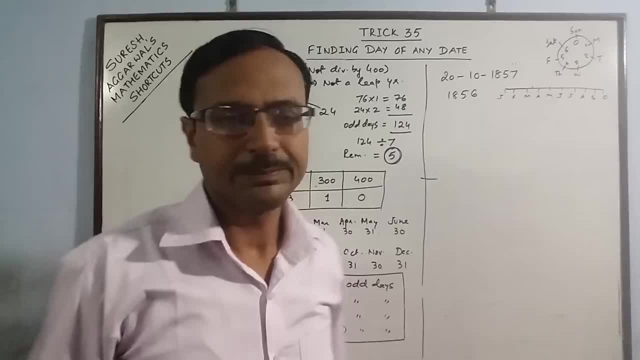 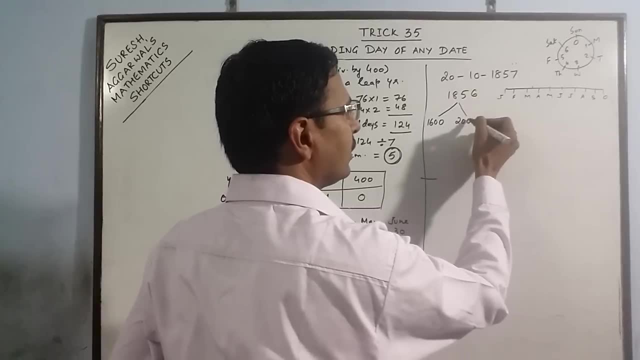 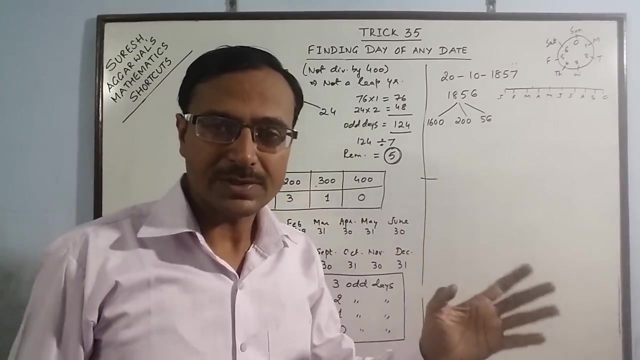 now 1856, complete years and one half year. This 1856 we divide into 1600, 200 and 56. Now see, I have divided into multiples of 400, because they can be only 1600 years, multiples of 400. 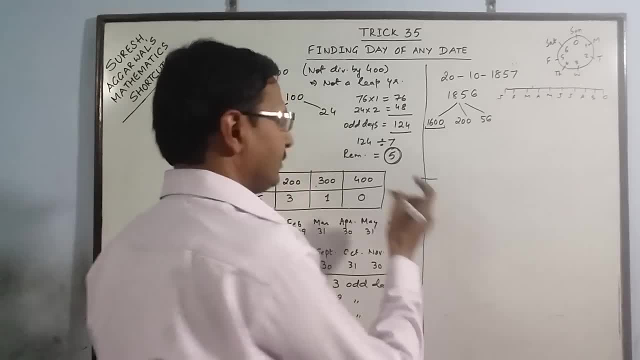 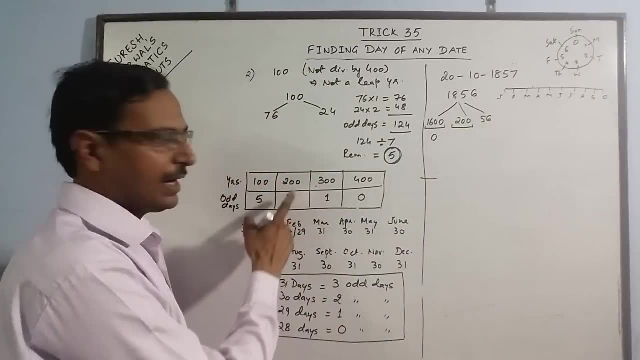 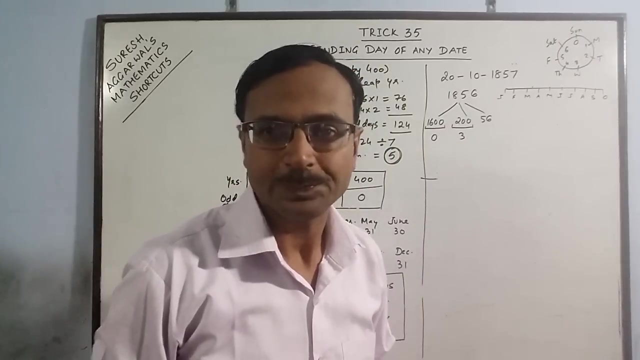 Every 400 years have 0 odd days, like here. So 1600 has 0 odd days, 200 have 3 odd days and for 56 years we have to find the number of lead years. now, 56 divided by 4 gives us: 14 and the remaining normal years 42.. So 42 and the remaining normal years 42. So 42 and 14.. Now for finding the odd days of this. this is normal year, So 42 into 1 and this. 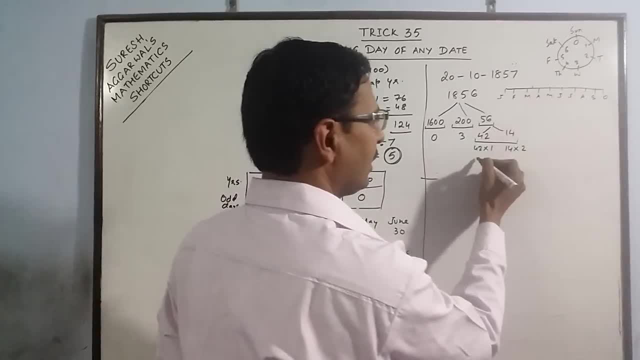 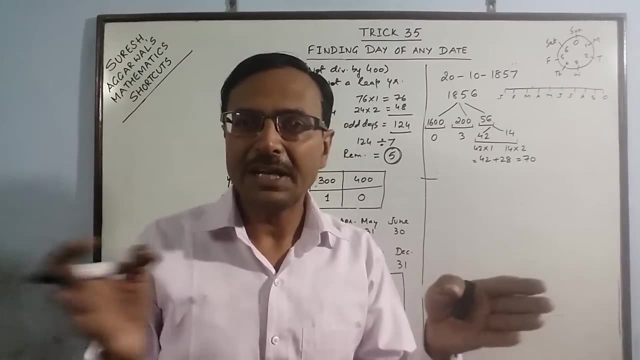 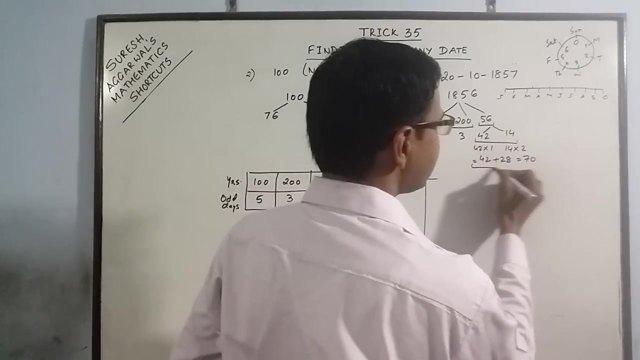 is leap year. Leap year has 2 odd days. So total 42 plus 28 gives us 70, and when you divide 70 into weeks of 777, then it is exactly divisible by 7.. So this is 0 odd days. So 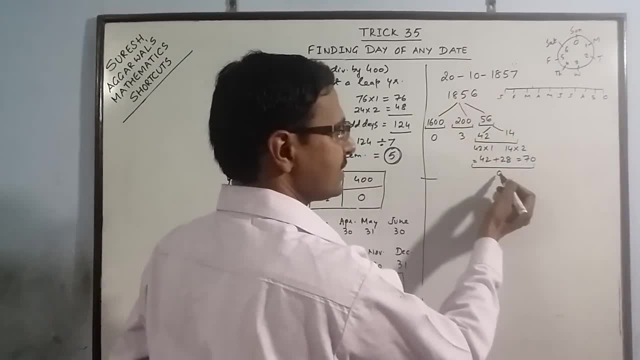 the total number of odd days is 0. So this is exactly divisible by 7.. So the total number of odd days in 1856 years is 0 plus 3 plus 0, that is 3 odd days. Now we have 3 odd days. 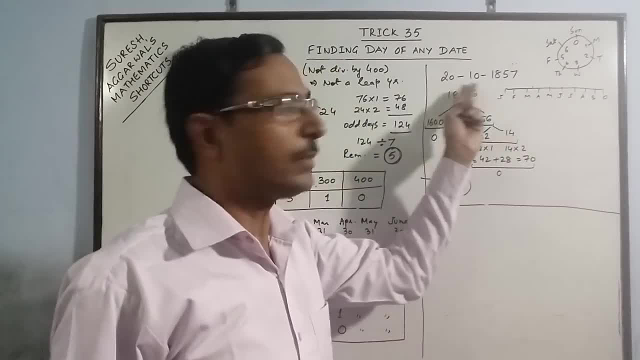 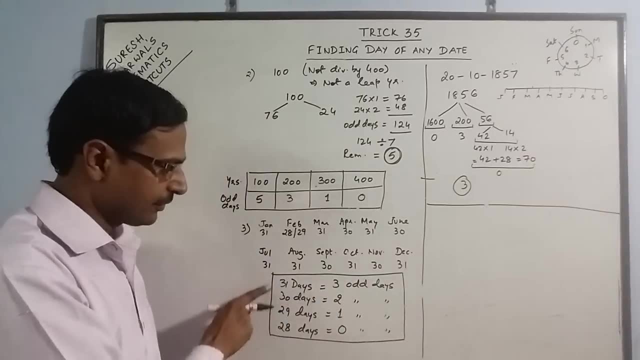 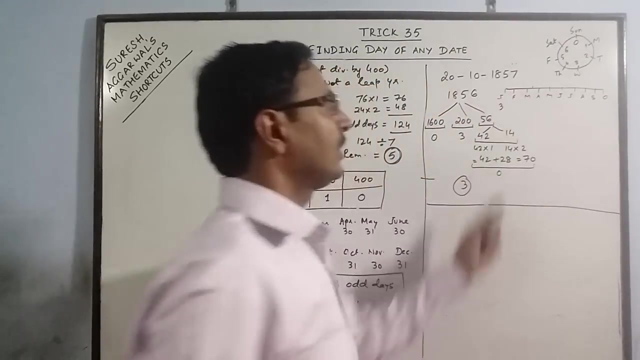 for this. Now come to the incomplete year. We have 31 days, January. I told you just now here the number of odd days for each month, January, is 31.. So 3 February Now this 1857 is a. non-leap year not divisible by 4.. So this is the number of odd days for each month. January is 31.. So 3 February. Now this 1857 is a non-leap year, not divisible by 4.. So 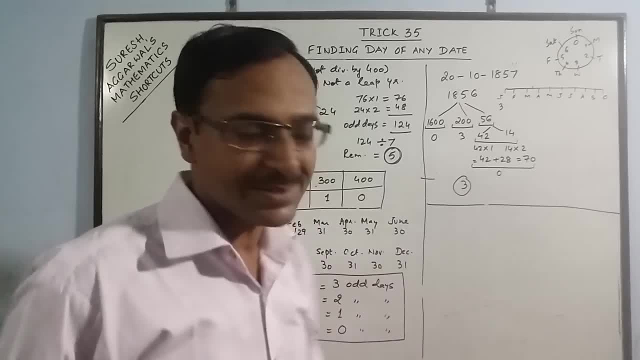 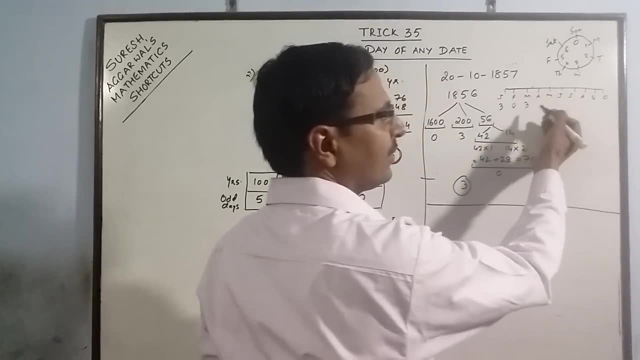 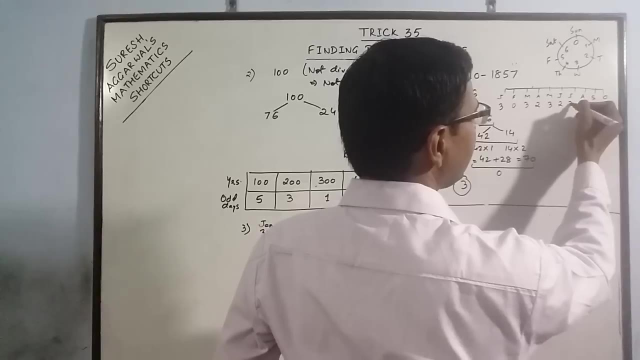 And in long leap year you have 28 days. So 28 days has 0 odd days: 0,, 3,, 31.. 30 means 2.. Then 31 means 3., 30 means 2., 31,, 3., 31,, 3., 32.. And October we have 20 days. 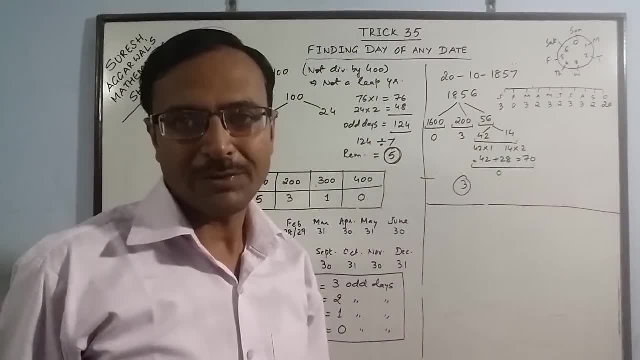 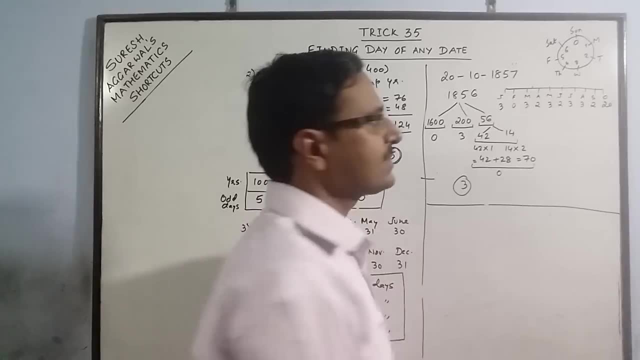 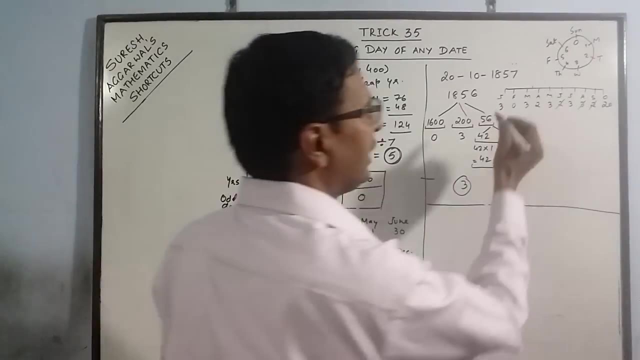 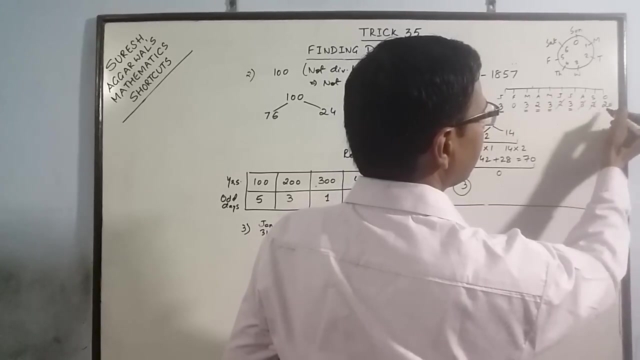 34.. Now these are the total number of days. You can cancel out 7s from here, because 7 constitute 0 odd days. 2 plus 3 plus 2 is 7.. So I have cancelled out 7.. Remaining 3,, 6,, 8,, 11,, 14,, 34.. 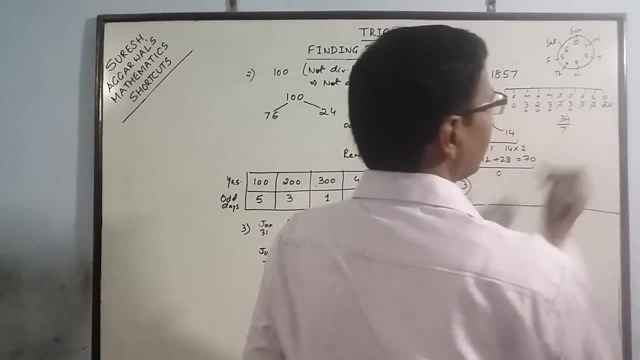 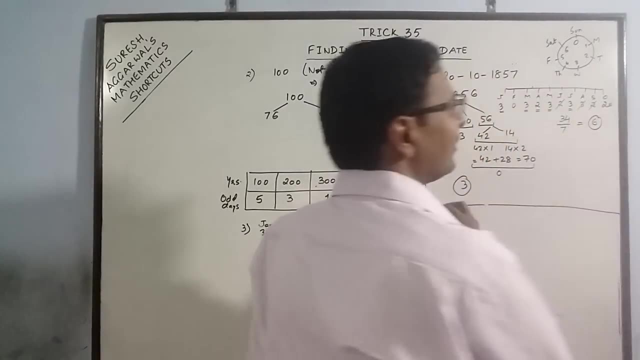 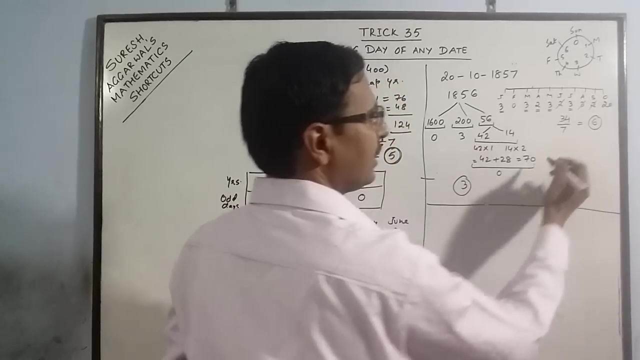 So 34 divided by 7.. Complete weeks: 7 fourths are 28.. So remaining 6.. So you have 6 odd days up to 20th October of 1857.. 6 plus 3.. Total odd days is 6 plus 3, 9.. 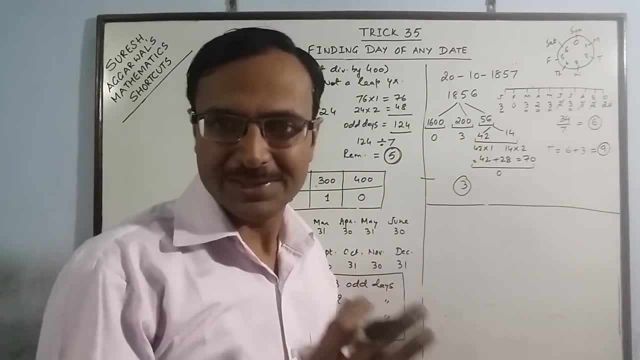 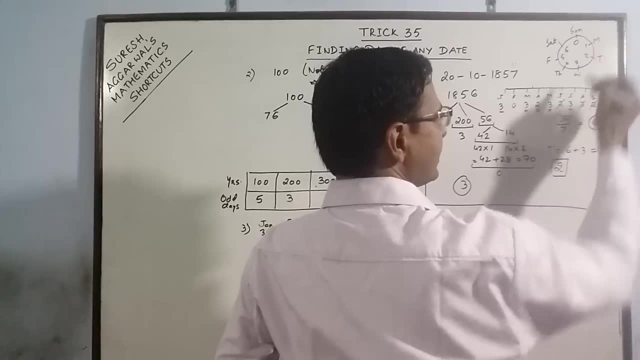 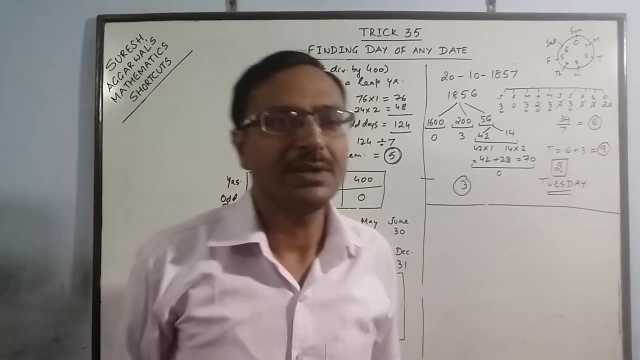 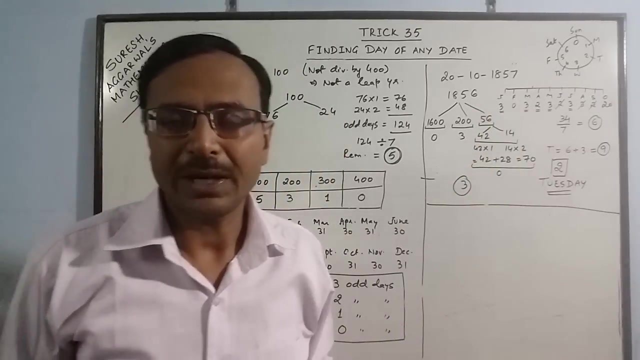 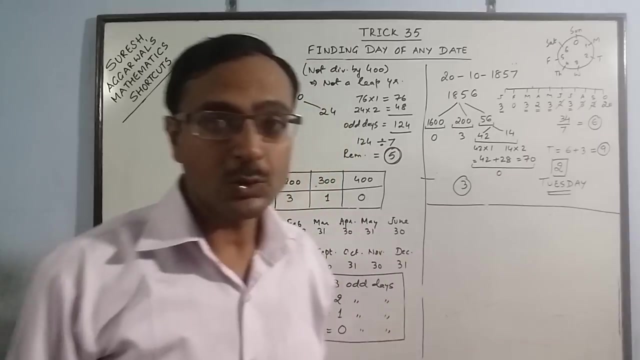 Again. divide this into weeks, So you have 7 plus 2.. So 2 odd days, And in this circle for 2 odd days you have a Tuesday. So a 20th October 1857 was a Tuesday. Seems a bit complicated, obviously, But you have to practice at least 8 to 10 problems of this kind so that you can grasp this trick and reduce your speed also. 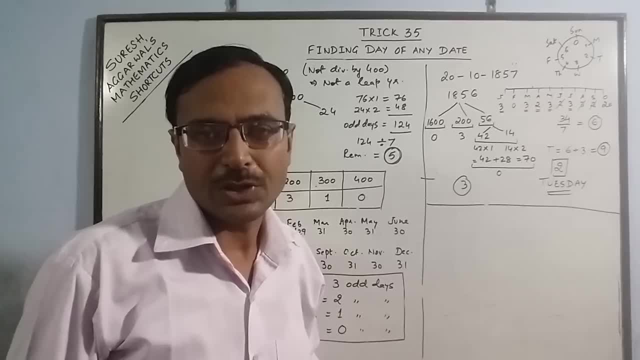 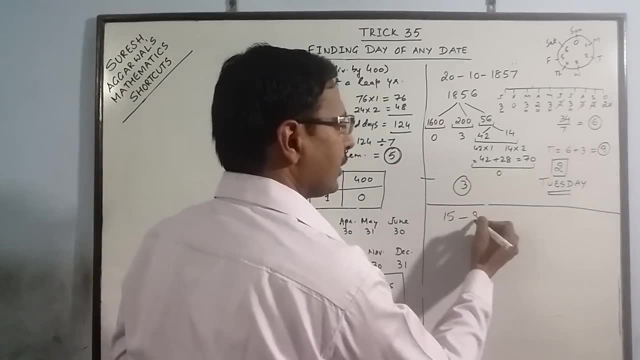 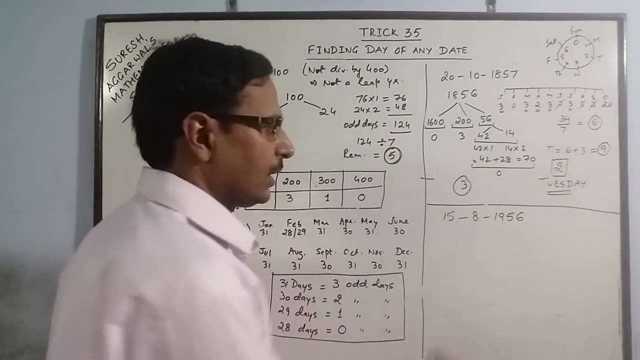 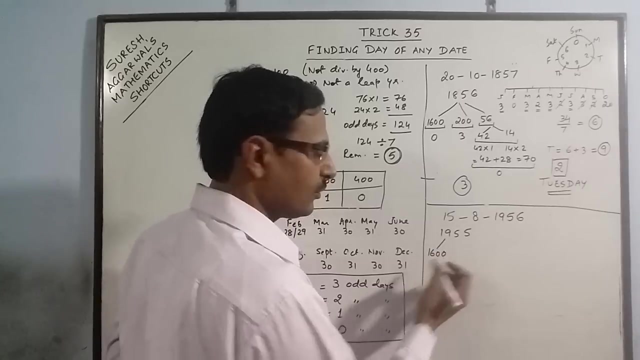 Now reduce your timing for calculation of this. Now let us take one example of a leap year. Say we have 15th October 1857.. This is a particular leap year, say 1956. Now here 1956 is incomplete. So we have 1955 years divided into 1600 multiples of 400. 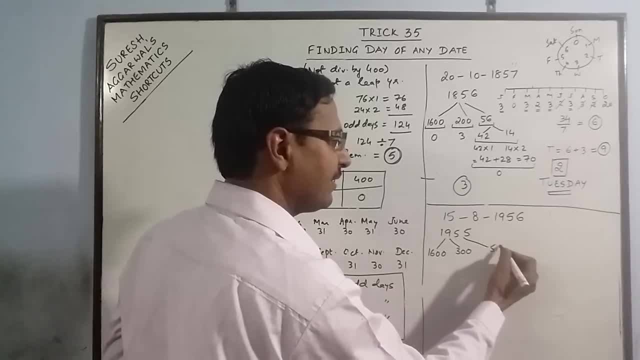 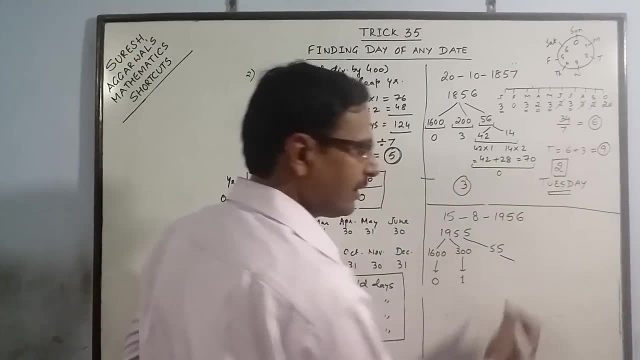 Then multiples of 100, 300 and 55. This is 0.. And for 300 years you have 1 odd day, 55, to be divided by 4.. So 4, 1,, 4, 3.. 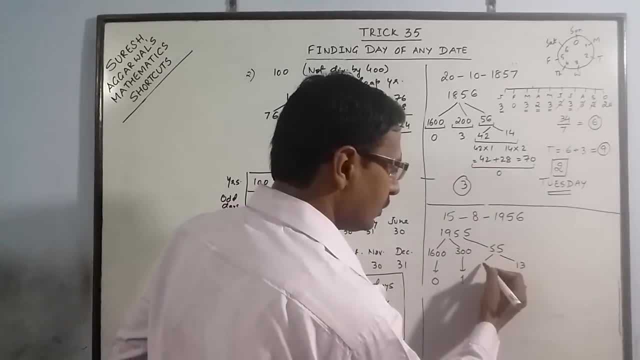 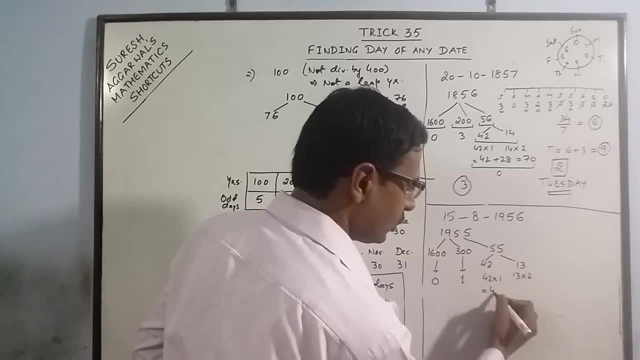 So 13 leap years And remaining 42. Normal years: Normal years: 42 into 1. Leap years: 13 into 2. So odd days: 42 plus 26.. 68. And when you divide 68. Divide by 7.. 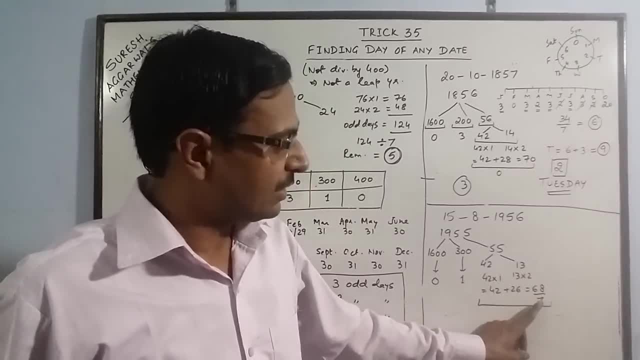 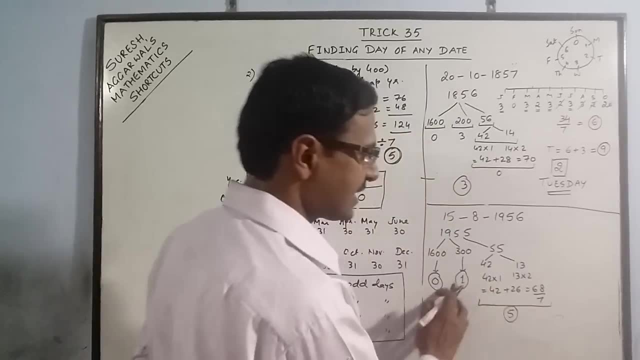 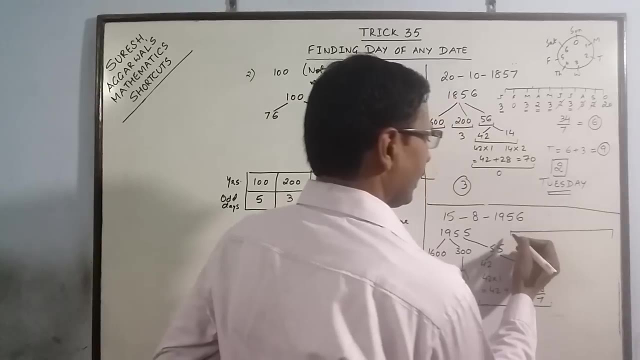 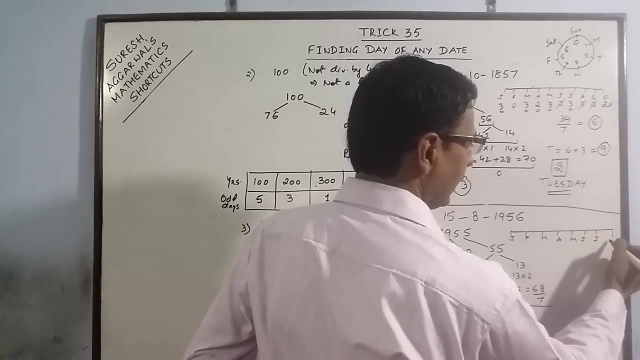 You get 7. 9 to 63.. So 5 remainder. So 5, 1 and 0.. So total: 6 odd days up to 1955.. And come to the month now, January, February, March, April, May, June, July and August. 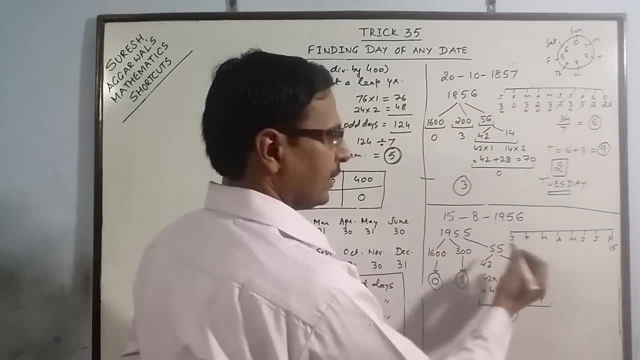 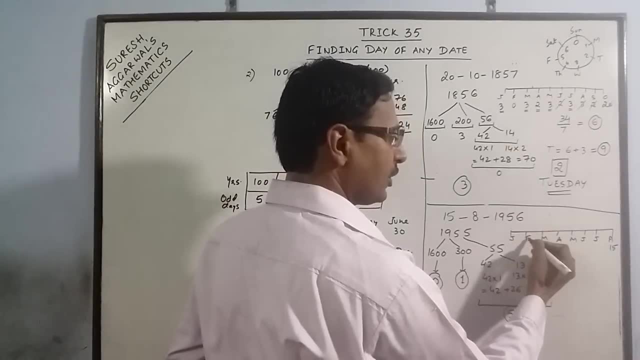 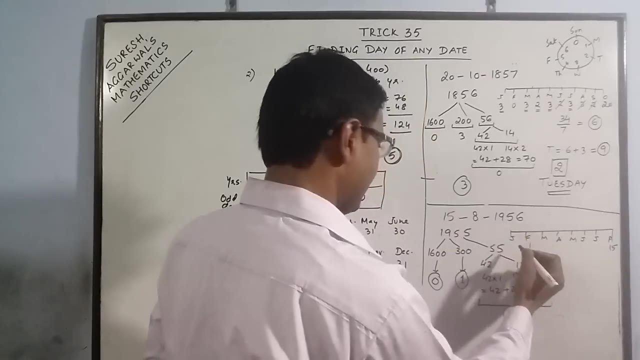 Because we have August here, So in August we have 15 days Remaining. according to this, 1956 is a leap year, So here in February you have 29 days, So 1 odd day. This is very important. January 31, 3 odd days. 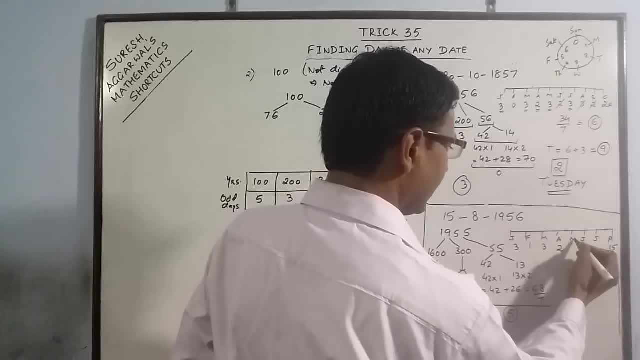 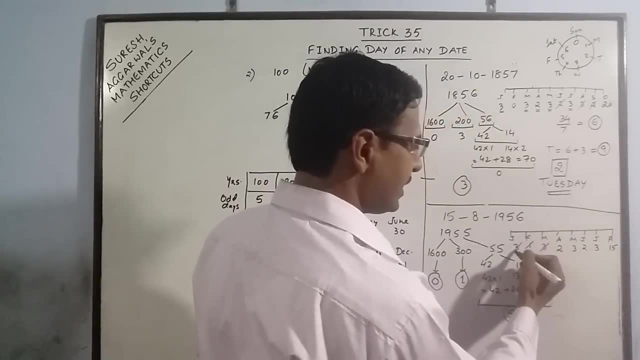 31,, 3. 32. 31,, 3., 32., 31,, 3.. Now cancel 7s. 3, 1, 3 is 7.. 3, 2, 2 is 7.. 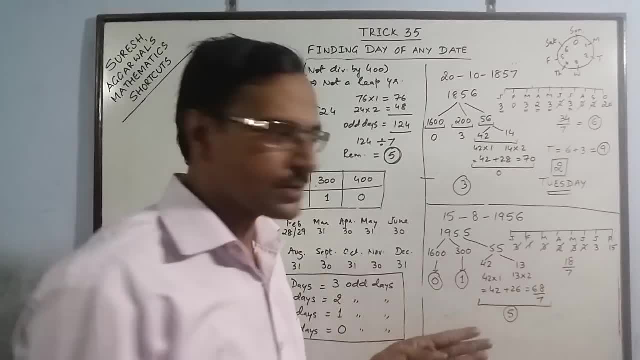 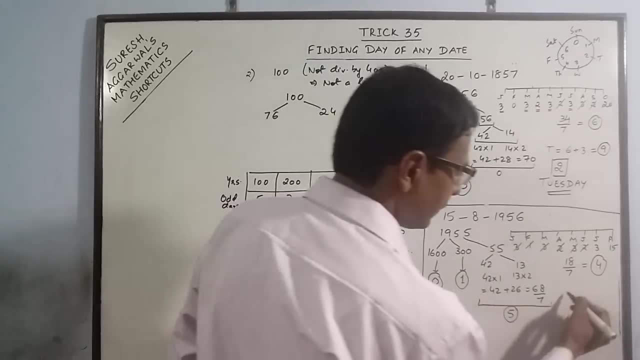 Now 18. when you divide into weeks, 7 to the 14 goes And remaining is 4.. Now total number of odd days: 4 plus 5,, 9 plus 1, 10.. 10 odd days: Again, it is more than 7..